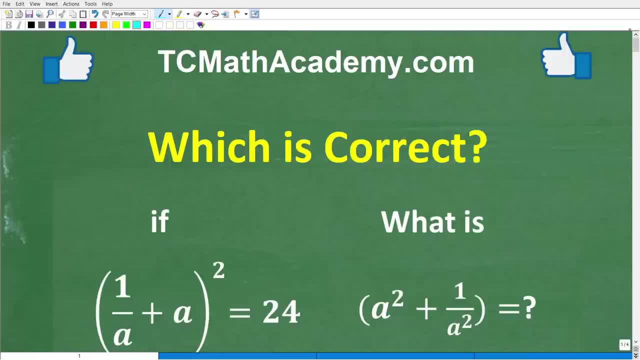 right answer in just one second. Then, of course, I'm going to solve this problem step by step, But before we get started, let me quickly introduce myself. My name is John and I have been teaching middle and high school math for decades, And if you need help learning math, check out my math help program at tcmathacademycom. You can find a link to that in the description below, And if this video helps you out, or if you just enjoy this content, make sure to like and subscribe, as that definitely helps me out. All right, so one more time. 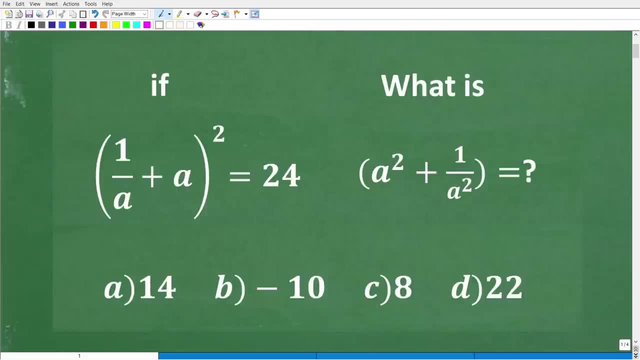 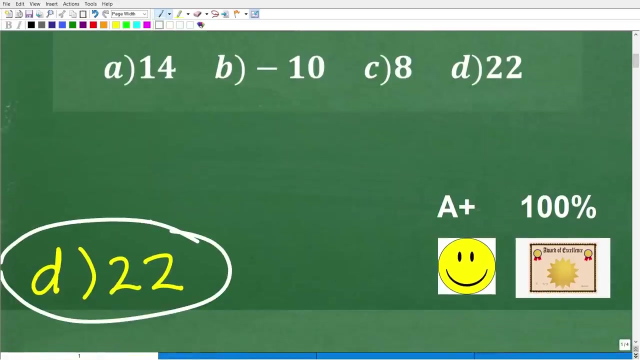 here is the problem, And you know it is designed to be a bit confusing. So if you're confused or if you're like I'm not quite sure what's going on, Well, that is kind of the design of the problem. But again, don't give up. right, If you have some basic algebra knowledge, you should still be able to figure this out. But let's take a look at the right answer. The correct answer is D22.. All right, now, if you got this right, you definitely get a happy face, an A plus and 100% and a Certificate of Excellence. 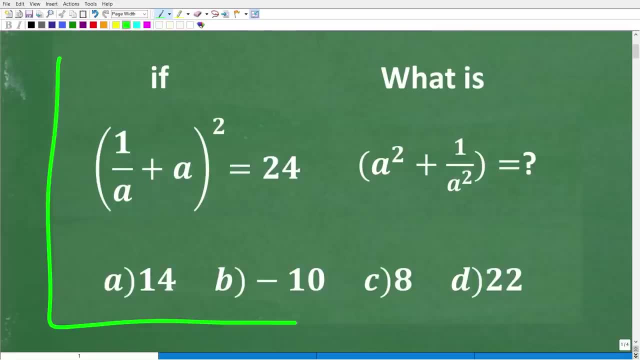 For being able to solve interesting and challenging and unusual math problems. So what I mean by unusual it's basically we just don't have like an equation here like right to x plus one is equal to nine. solve for x. this is not a typical type of, let's say, math or algebra homework problem or something that you would even see maybe on a you know, kind of like a chapter test. So you do have to think about this from kind of maybe a different perspective. But let's 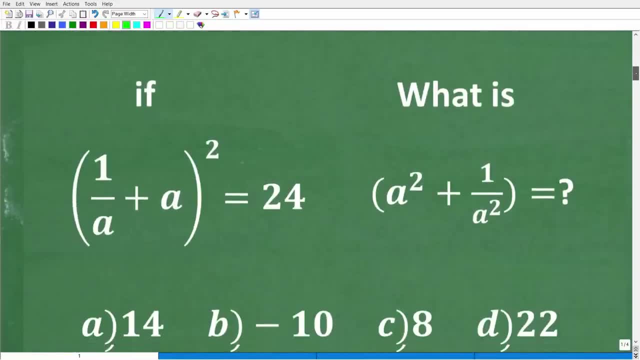 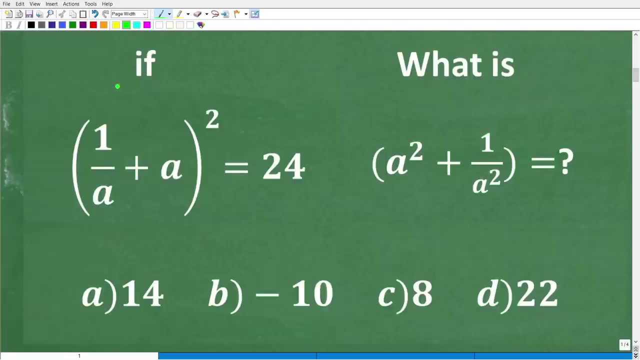 go ahead and get into the solution And if you didn't get this right, well, let's cover this right now. All right, so here is our problem, And it's kind of like a two piece problem, right? So it says: if we have this, then what is this thing over here equal to? Now, let's suppose the problem was: 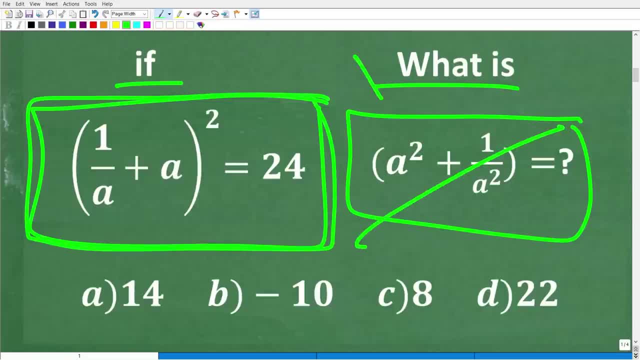 solve this equation right here, right? So let's just forget about this. for a second- And this is a multiple choice question- you could be like: Oh well, I'm looking for what A is equal to, So I can just test these values, even if I don't know how to solve this equation and figure. 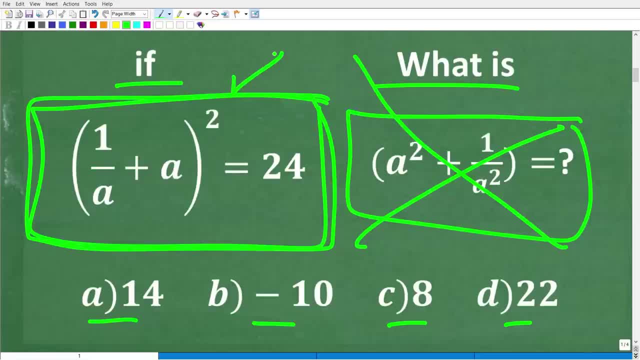 out. you know what is the right solution to this equation. But that's not the problem, And that's what makes this question a little bit unusual. The problem is: hey, what is this thing, right here, equal to in value, right? So we know, we know that A squared plus one over A squared is equal to 22.. 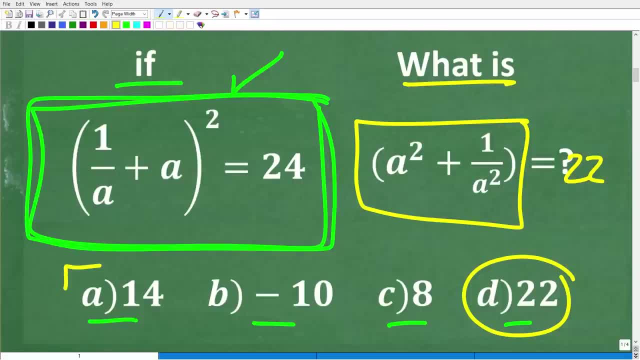 So what do we, you know, face with here? Well, our answers are really not going to help us too much, But well, in some respects, you know you could, you know maybe, say: well, this is equal to 22.. Of course, you don't know that because I'm telling you the answer, But if you're looking at 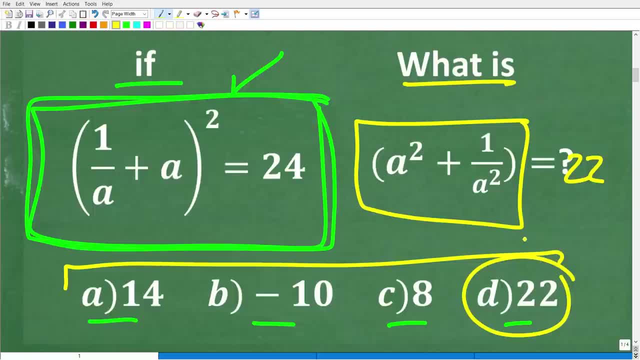 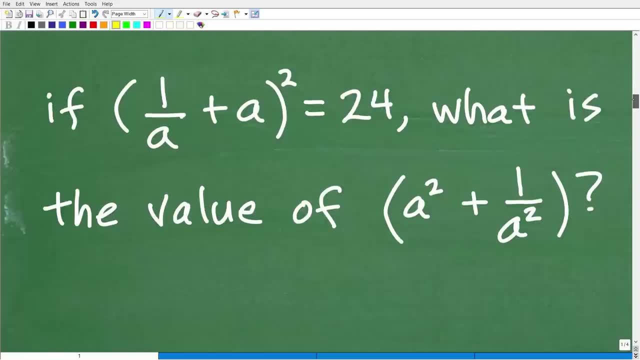 the question. you're like: well, I really don't know what to do. Well, you know, that's again what makes this problem a little bit challenging. So let's go ahead and talk about this problem right now And think about it from this standpoint. So if parentheses one over A plus A squared, 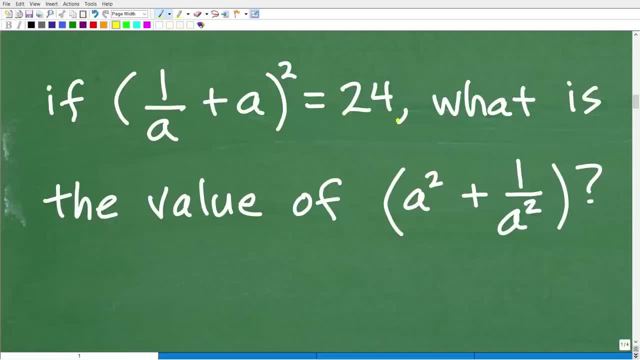 or my sorry parentheses, one over A plus A and C squared is equal to 24.. What is the value of this? Well, what we have here is this variable, A right, So, and of course, we have an equation. So you might be saying to yourself: well, maybe. 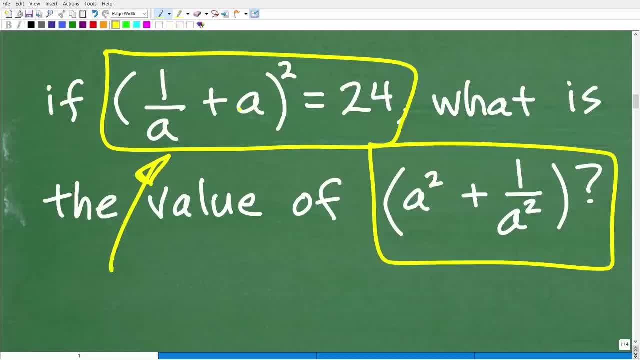 we have no alternative but to figure out what A is equal to, because if we can figure out what A is equal to the numeric value of it, so maybe, like, A is equal to three. Well, if we can solve this equation and figure out the solution, then we can plug it in over here and get the value. 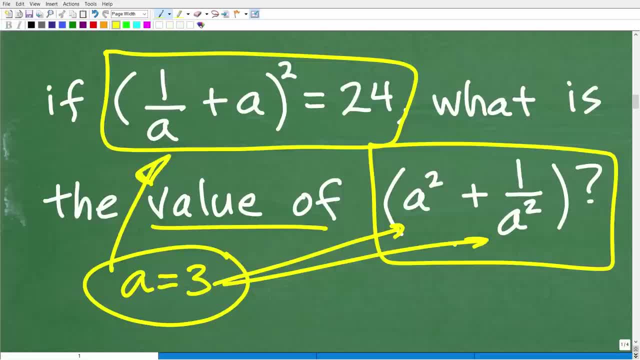 of this expression And really that's what we're going to have to do because there's really no other good options. But if you're out there and you're like saying, hey, Mr YouTube, Math Man, I know another approach to this, Well, that is fantastic. Again, there's often more than one way to solve. 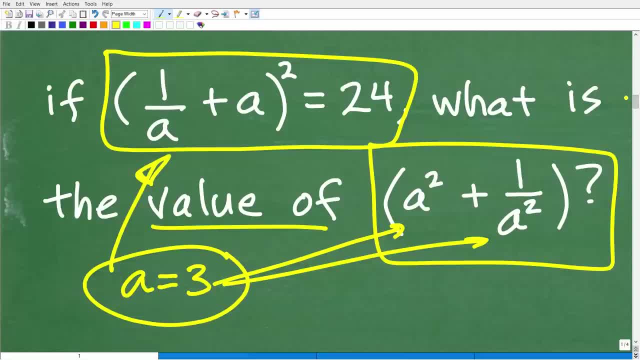 a problem. But let's go ahead and just follow this strategy And that is, let's solve for A in this equation and then get that solution, And then we can kind of plug it into here and get the right answer. So let's go ahead and do that. 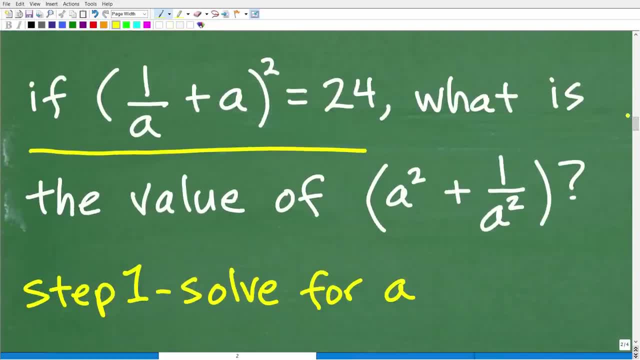 So this is going to require some algebra, All right. So if our equation right here is equal to 24, what is the value of this thing? So step one is going to be solve for A in this equation, because we do have an equation and hopefully, you know, we have the algebra skills to solve. 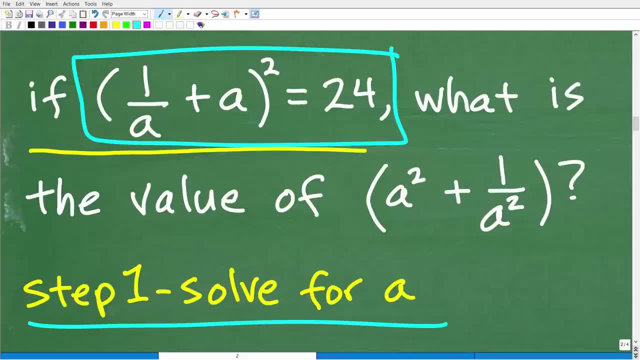 this equation, But remember, OK, you have to. I'm giving you a big hint here. The question is: what is the value of this expression right here? A squared plus one over A squared, All right. So this is a big hint, And let's go ahead and start. 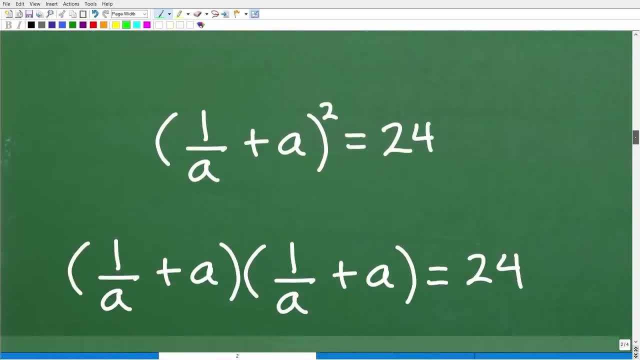 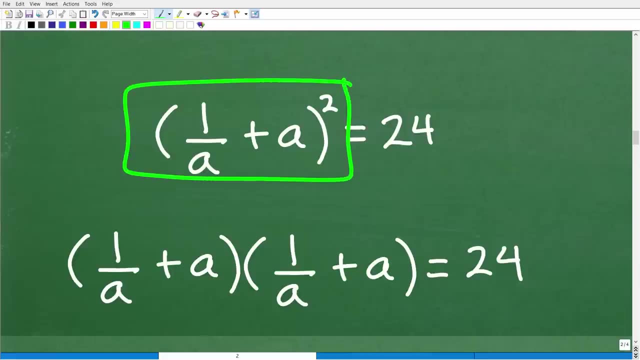 this process now. So let's solve for A. And what do we need to do? Well, we have no choice but to expand this expression right here. So we have one over A plus A, in parentheses squared. So this means take one over A plus A and multiply by itself. Right, That's what it means to square. 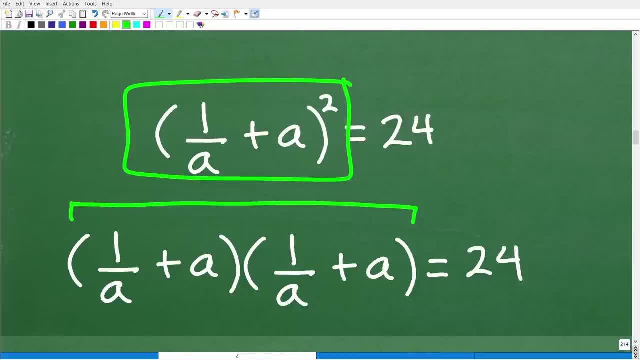 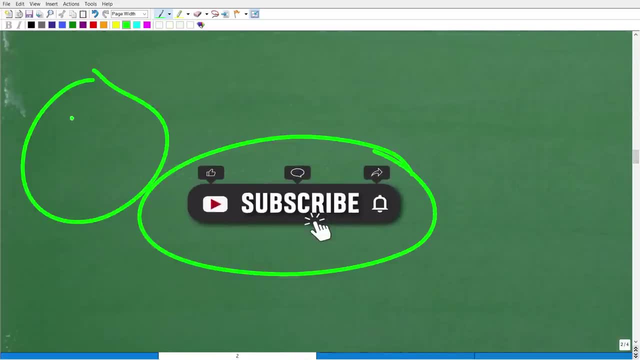 this. So let's do all this algebra and then see where this problem takes us. But let's take this next step, And that is quickly subscribe to my YouTube channel Now, if you enjoy mathematics. but some of you are like: hey, what are you talking about, Mr YouTube Math Man? I don't. 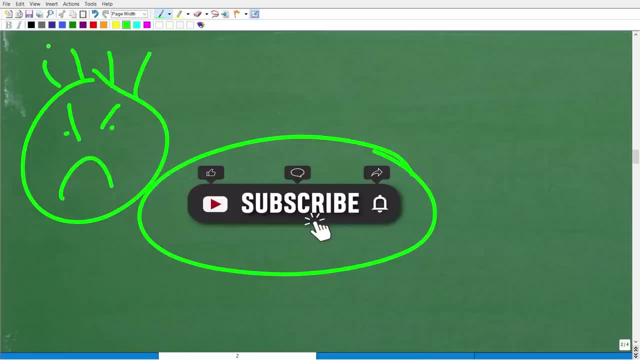 really enjoy math. I just come to your channel just to try to figure out how you know how to do my homework or get ready for a test. Well, that's perfectly fine as well, because my channel is all about trying to make math clear and understandable, But I need your help in order. 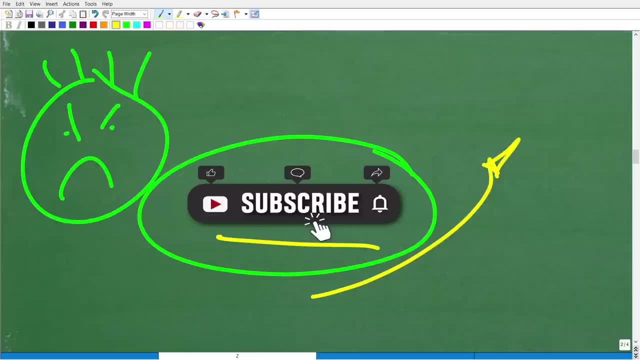 to reach as many people as possible. That's just not going to happen on its own And YouTube really consider how many people you know subscribe to my channel. So it really does help me out And hopefully you might be saying: all right, Mr YouTube, Math Man, just so you can get to the rest. 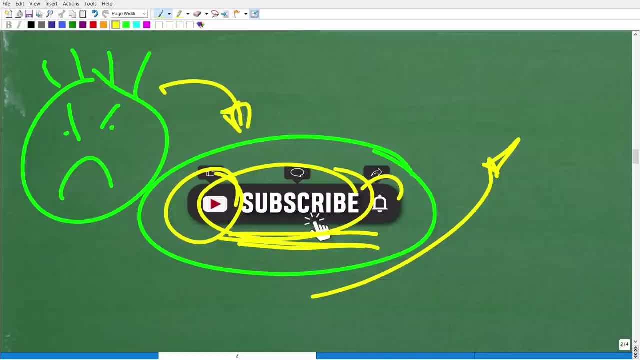 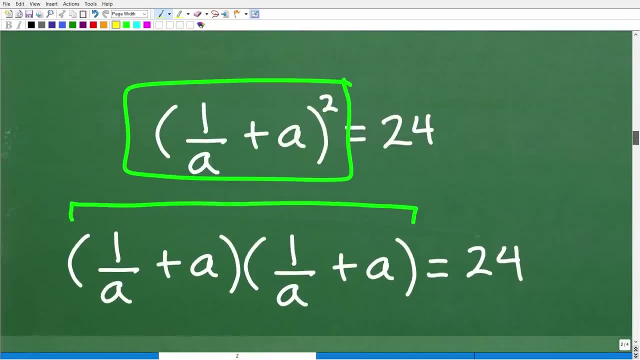 of the solution here. I'm going to subscribe and I'll be like perfect, But make sure you hit that notification bell as well so you can get my latest videos. All right? So let's go back over here before we really get into this problem And I want you to focus on the question. So we have this. 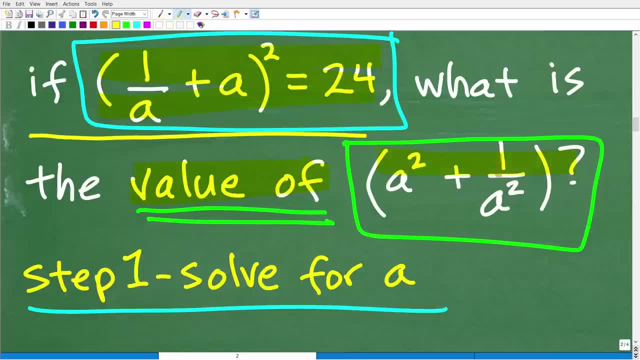 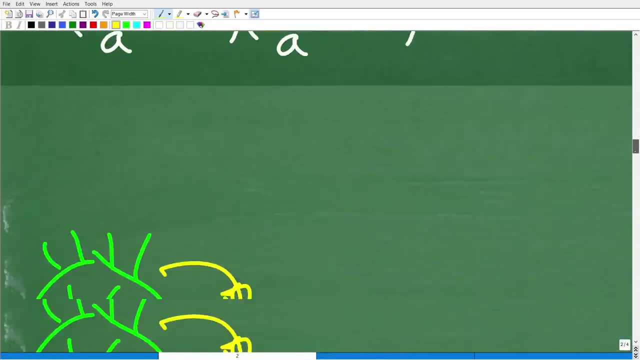 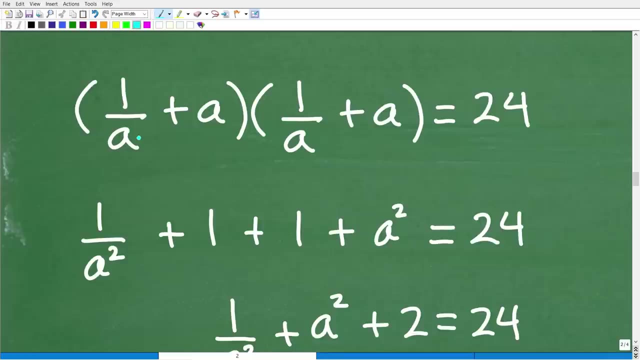 question: What is the value of this thing right here? What is the value of a squared plus one over a squared? All right, So let's go ahead and get into this algebra right now. All right, So here is what we need to do: We need to multiply these two binomials, So we're going to use the FOIL. 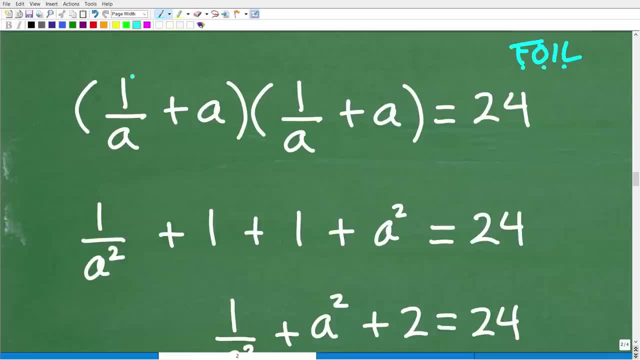 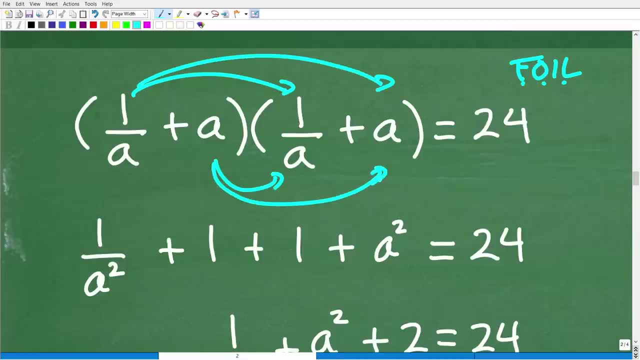 method F-O-I-L: first outer, inner, last. So we're going to multiply this times: this, That's the first terms, And then we're going to multiply the outer terms, And then we're going to multiply the outer terms. Now, if there's anything in here that you don't understand from an algebra, 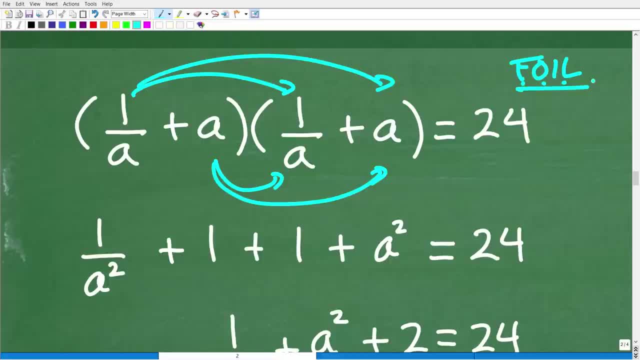 perspective. check out my full main math courses- You can find links to those in the description of this video- or check out any one of my 3,000, well, not any one, but I have like 3,000 videos on my. 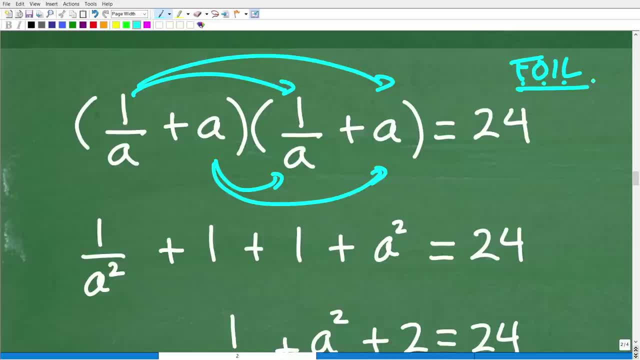 YouTube channel from basic math to more advanced math, And I'm pretty sure I cover how to multiply polynomials and binomials in some of my videos. Matter of fact, I don't even I've done so many videos. I pretty much covered a whole wide span of things, But if you want my best instruction, 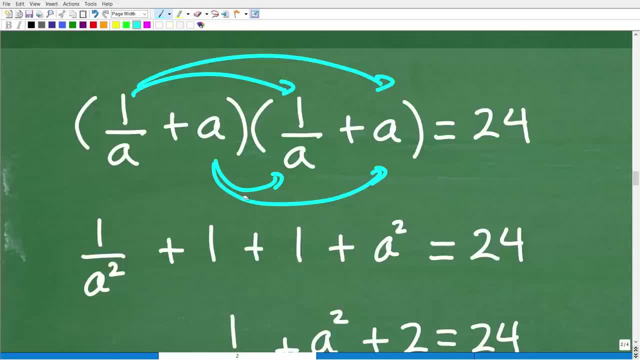 check out, like my YouTube channel, and I'll see you in the next video. So let's go ahead and do this multiplication And we'll take it nice and slow, because we do have some fractions here. So 1 over A times 1 over A is what? 1 over A squared right? So that's 1 over A. 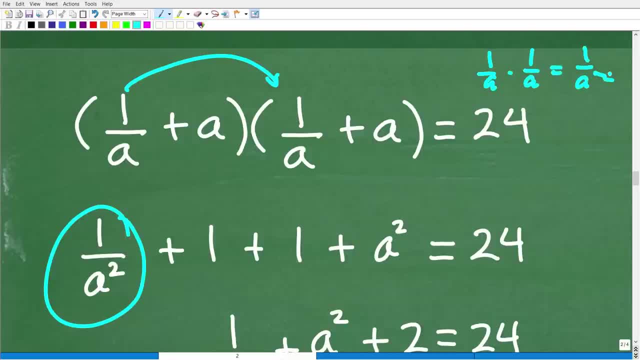 times 1 over A, So we're multiplying fractions. That's 1 over A, squared. All right. So 1 over A times A is what? Well, 1 over A times A over 1 is going to be 1, right, So we're going to end up. 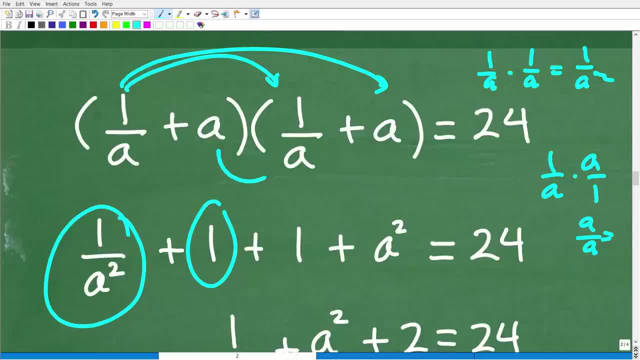 so 1 over A times A is 1.. Okay, So A times 1 over A, that's also going to give us a 1.. And then A times A is going to give us an A squared. All right. So that is the result of multiplying these. 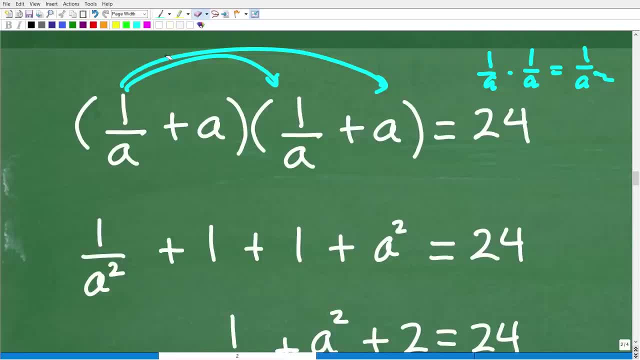 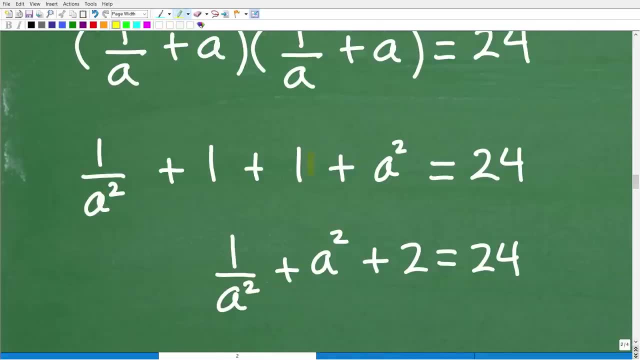 two binomials. We end up with all these terms right here, but we have to continue to clean this thing up. Okay, So we have 1 over A squared, plus 1 plus 1.. So this is obviously going to be 2.. 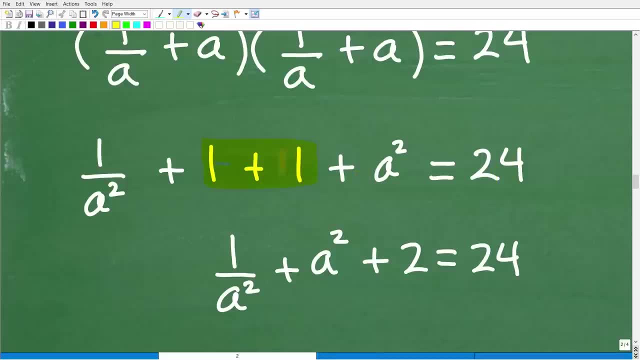 And then we have A squared is equal to 24.. All right, So we'll add the 1 over A squared, So that is 2.. So we have 1 over A squared plus A squared plus 2 is equal to 24.. All right, So. 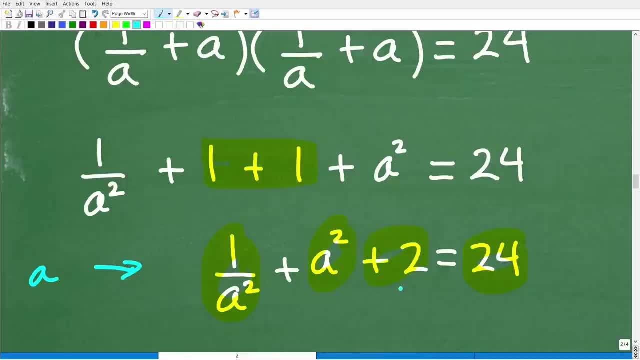 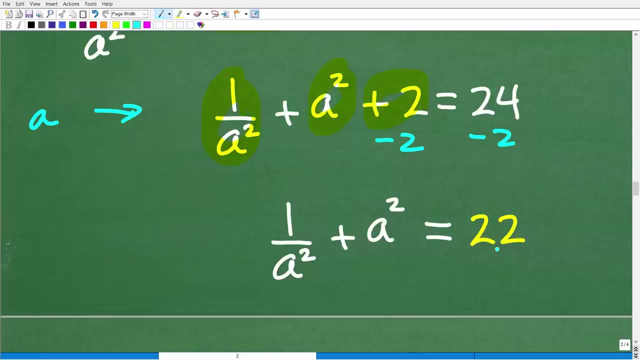 again, we're trying to solve for A, So let's go ahead and get 2 on the other side of this equation, And we'll do that by subtracting 2 from both sides of the equation, And when we do that, we get 1 over A squared plus A squared is equal to 22.. All right, So let's continue, But actually 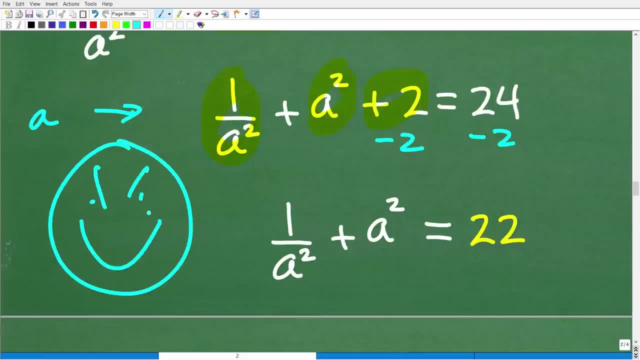 let's stop. This is where this problem becomes very sneaky. And you might be saying: what are you talking about, Mr YouTube? Math Man, Continue on so we can solve for A. Well, really, we don't need to do anything. And you might be saying: what are you talking about? Well, this is the answer to 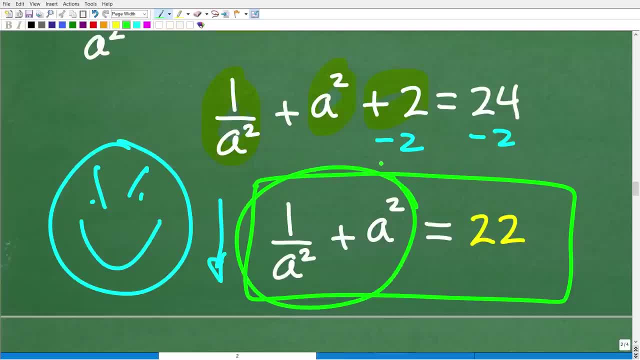 our question. Okay, Remember. the question is: what is the value of 1 over A squared plus A squared? Okay, Well, we just figured it out: This is equal to 22.. So let's go back to this question again. And I was saying: what is the value of 1 over A squared plus A squared? And 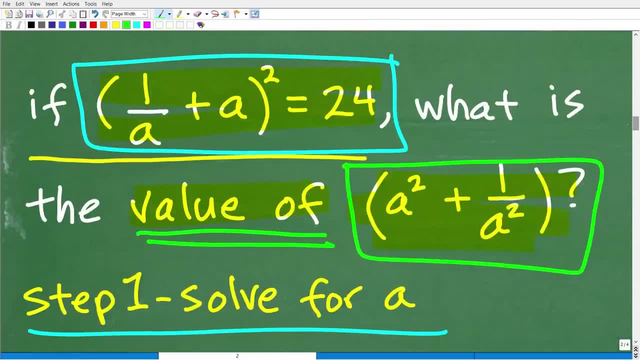 I was trying to give you a hint on it. So here it is. So if 1 over A plus A squared is equal to 24, what is the value of this thing? A squared plus 1 over A squared. So we kind. 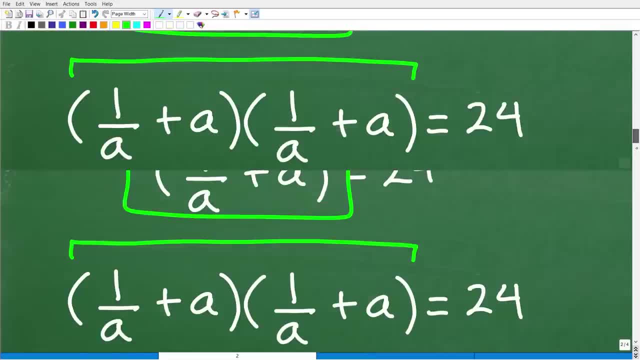 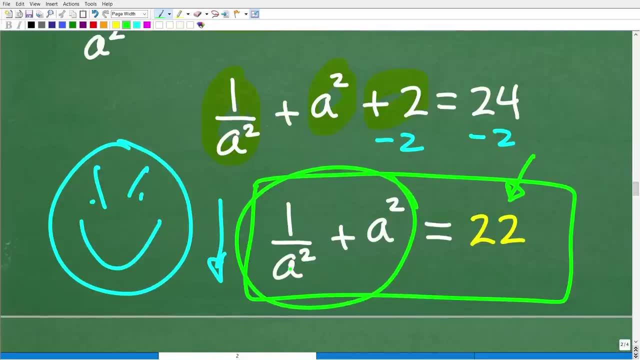 of have to be on the lookout for this expression, And we found it way over here. We found it as we're going through these steps. We kind of stumbled upon it. We're like, hey, what I mean here this is 1 over A squared plus A squared. We don't really need to continue. 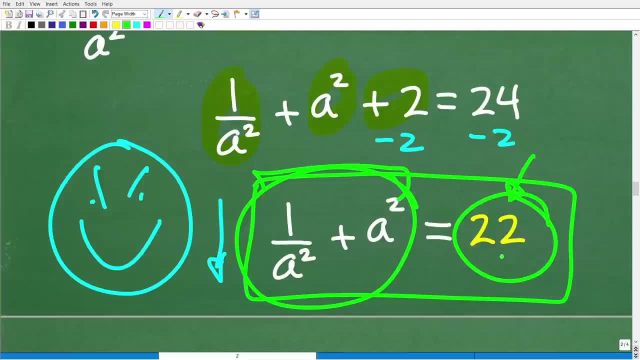 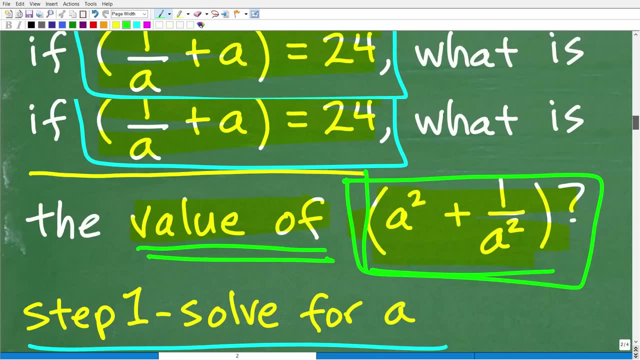 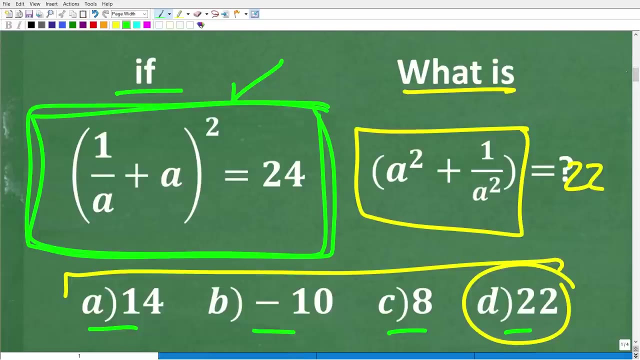 to solve for A, because this expression is equal to 22.. All right, So what is the whole point of this problem? Well, the point of it is that in mathematics, you're going to come across unusual type of situations, especially for those of you that still have to take exams like the SAT, ACT or any creative type of 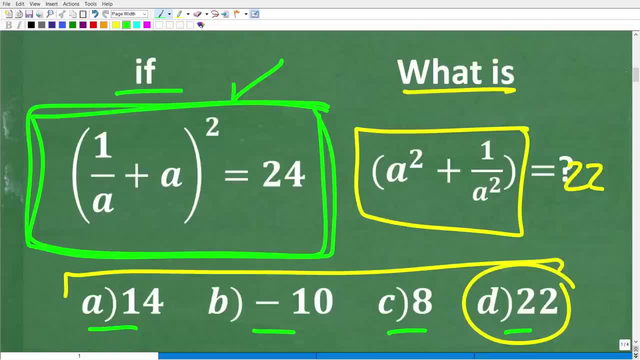 an exam, Let's say a math placement exam. It doesn't make a difference. If you're taking some sort of math exam and if you have a good teacher constructing those exams, they're going to challenge you on some type of problems. In other words, not everything is going to. 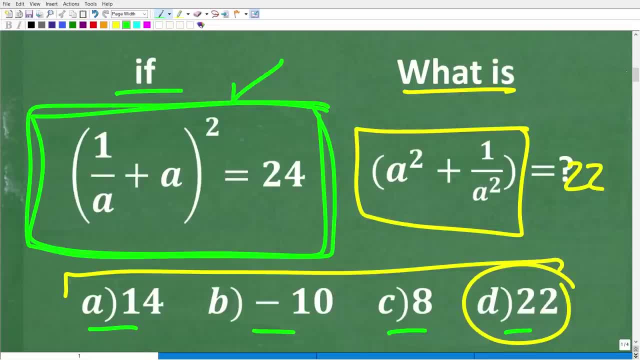 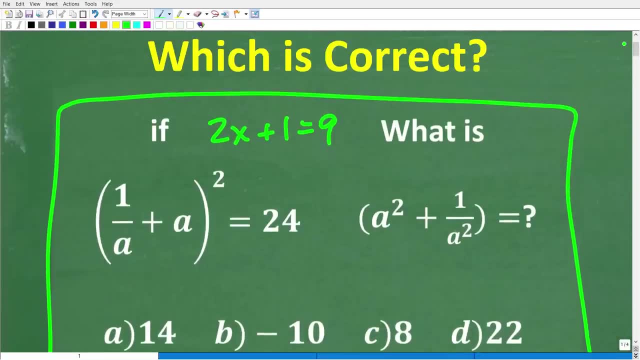 be so straightforward, But in this problem here you really have to focus on the question, And that is a big part of figuring this thing out. is focusing in on what the question's asking. Well, obviously we have an equation there that involves A, But really the question?